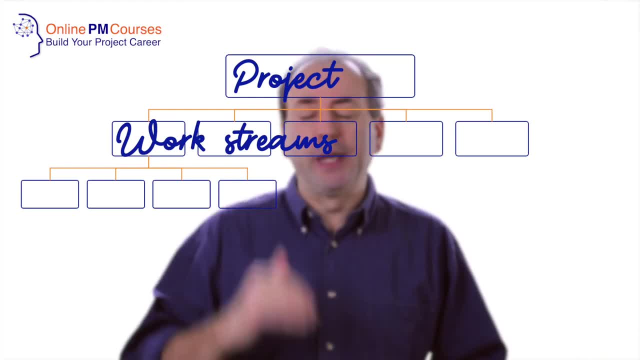 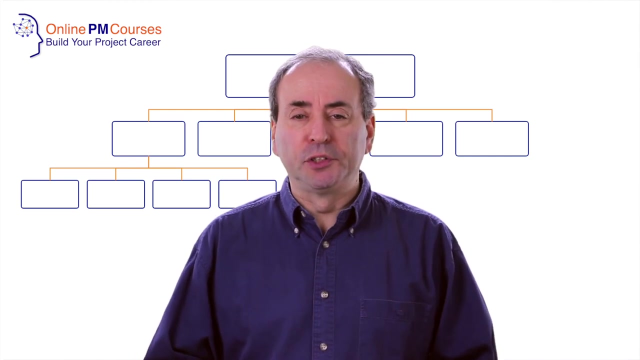 each of those principal components gets further broken down until we end up at the lowest level of the hierarchy, with individual tasks or activities that the person who will carry them out recognises as a single, coherent task that they fully understand. Now, the representation I've put on the screen is very useful for understanding a work breakdown structure. 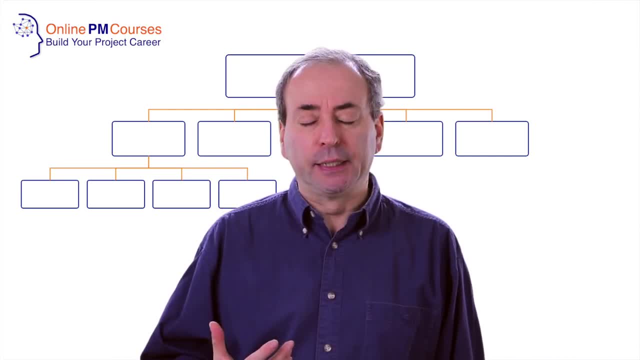 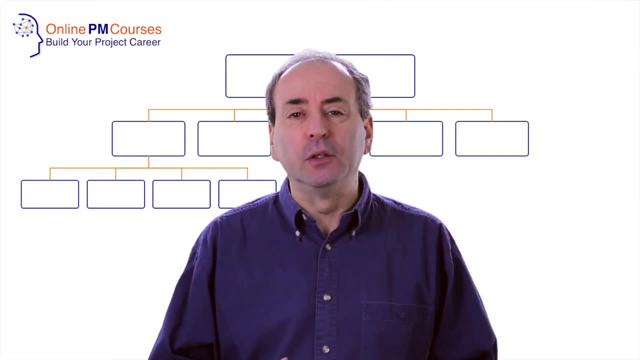 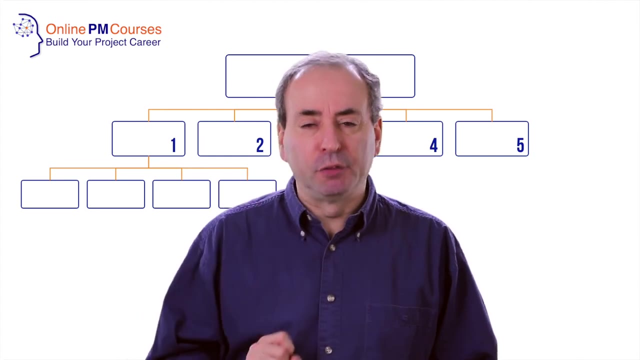 but it's absolutely rubbish for representing it across a large project. It will just rapidly get out of hand, And so what we actually do is we number across the principal activities and then, for each thing that flows from those activities, we give it a sub-numbering system, And so we 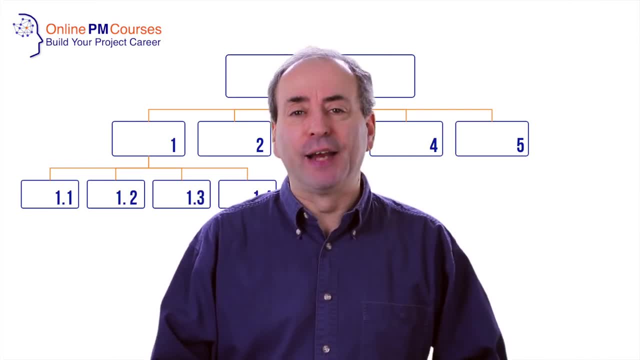 end up with a comprehensive list of every activity that needs to be done. the scope of the project. The proper way to plan projects is to develop your work breakdown structure before you start thinking about dependencies and sequence, which will, of course, give you your network chart. 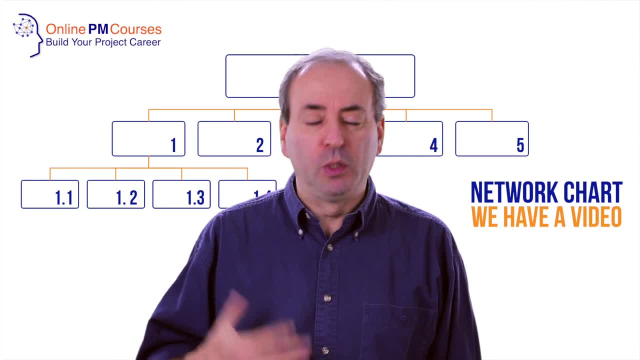 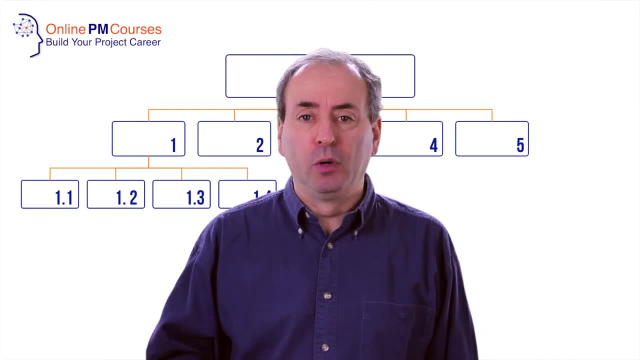 or elapsed times for each of the tasks, which will allow you to draw up your Gantt chart. The best way to produce a simple work breakdown structure if you're working on a small project is with a word processor tool like Microsoft Word. If you're working on a larger, more rigorous project, then you will no doubt have some. 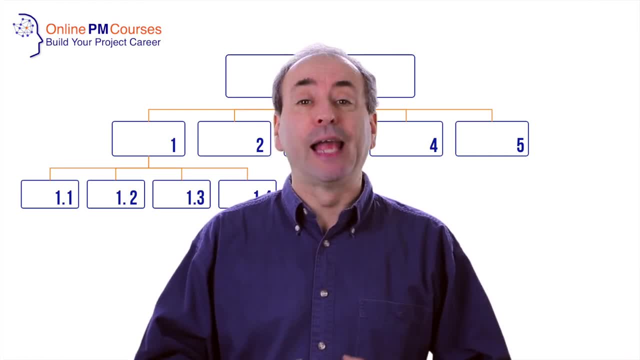 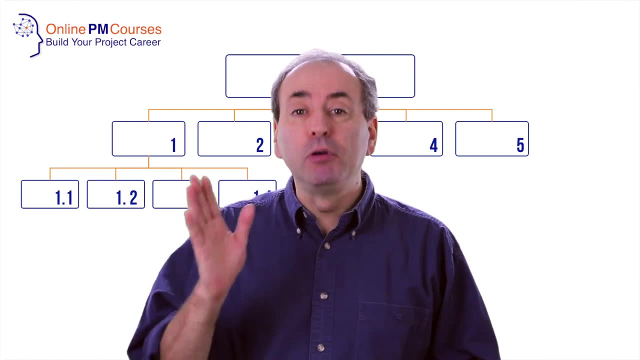 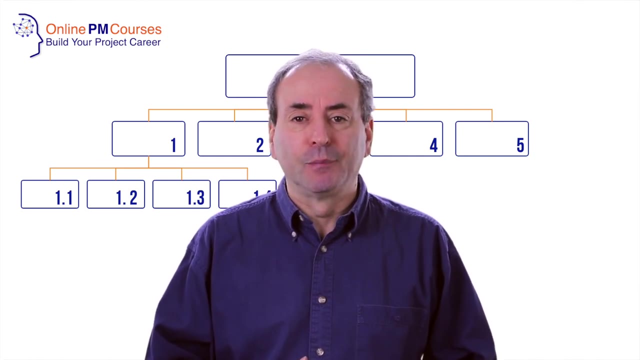 form of project management software that will allow you to capture every activity, allocate unique reference numbers to them and create your work breakdown structure as a preliminary step to producing your network chart, your critical path and your Gantt chart. Tools such as microsoft project are designed to do this. 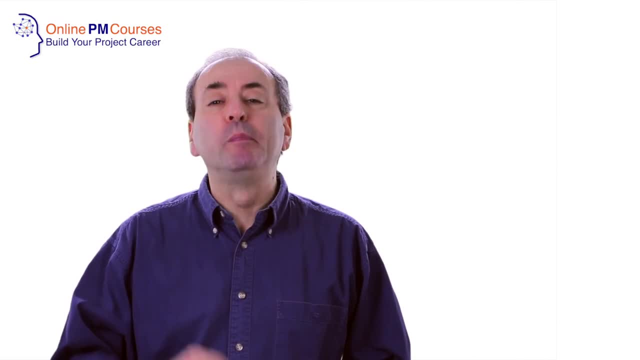 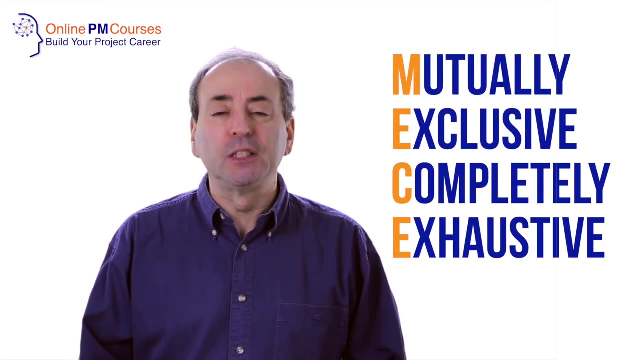 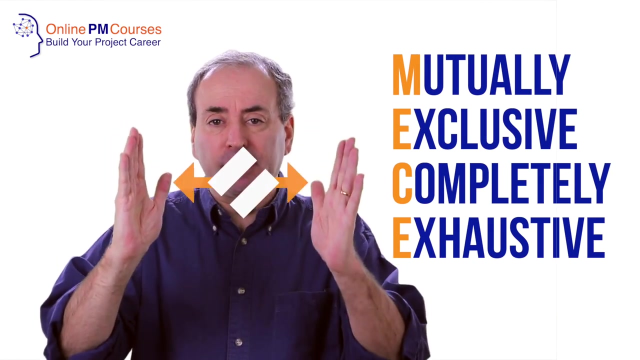 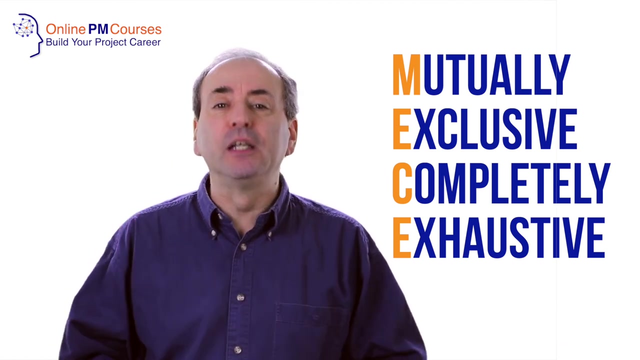 a good work. breakdown structure will be MECE, and that stands for mutually exclusive and completely exhaustive, that is to say mutually exclusive. each task is clearly distinct from each other task. there is no overlap between the tasks, and completely exhaustive means that everything you need to do on your project. 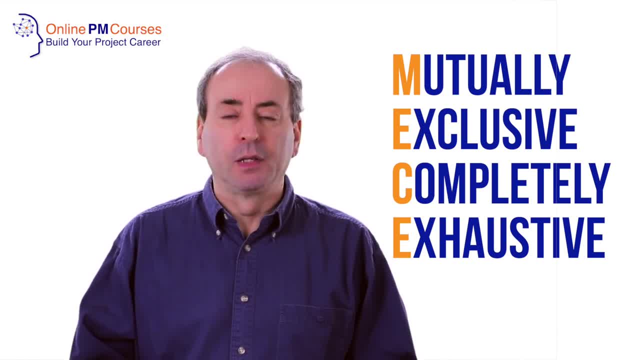 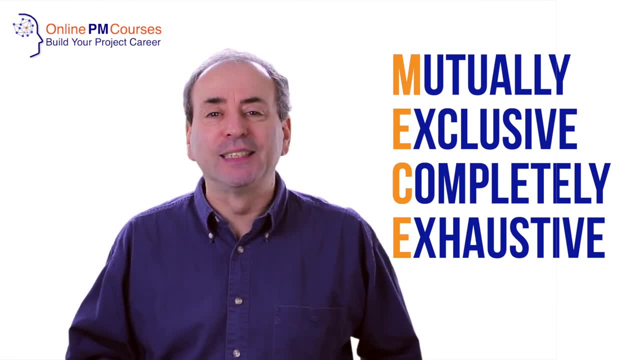 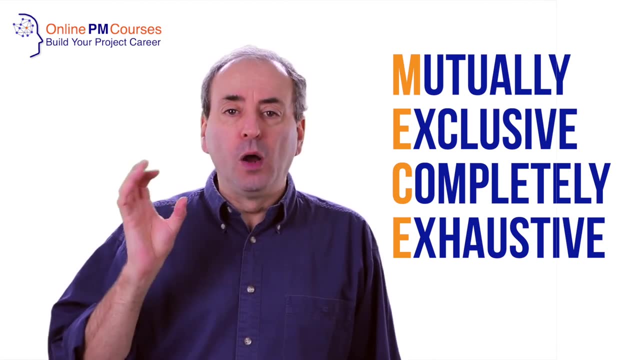 is covered on your work breakdown structure. the thing that many project managers miss out of their work breakdown structure are all the tasks and activities concerned with managing the project. so, as a matter of habit, i will always create one work stream, one major area of work on my work breakdown structure, labeled project management. 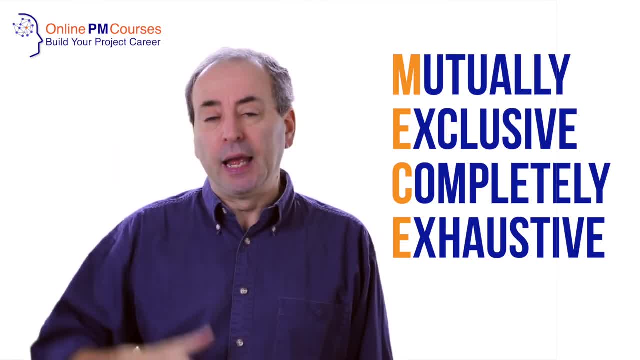 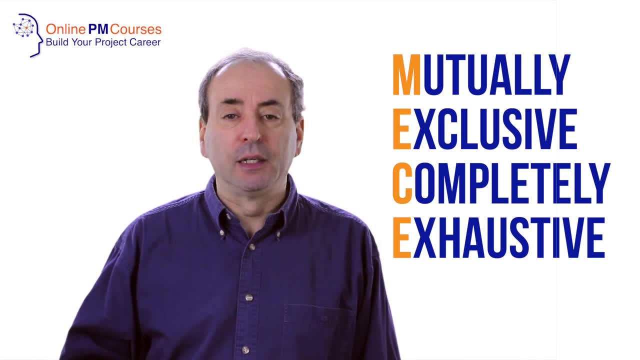 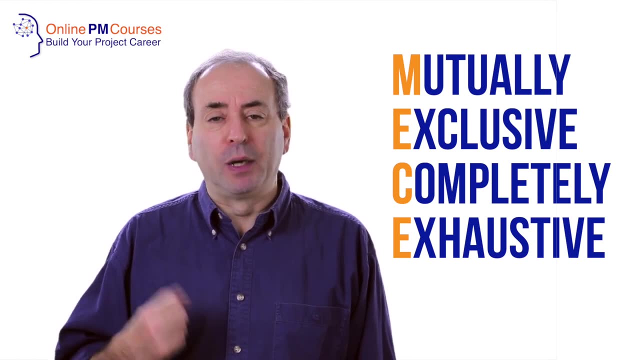 that way i capture all the tasks it takes to manage the project and then when i start budgeting the project and allocating resources, i have those tasks ready to budget and resource and that ensures that i don't forget the project management activities and i've got the budget and the 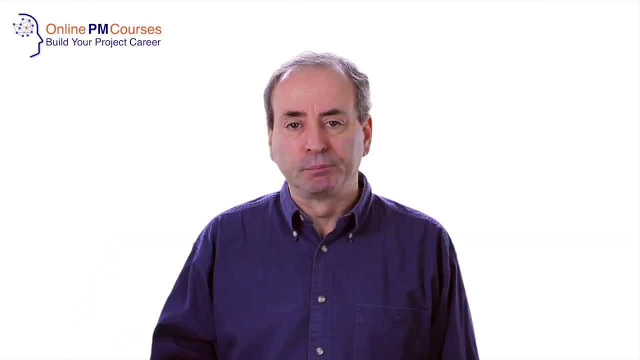 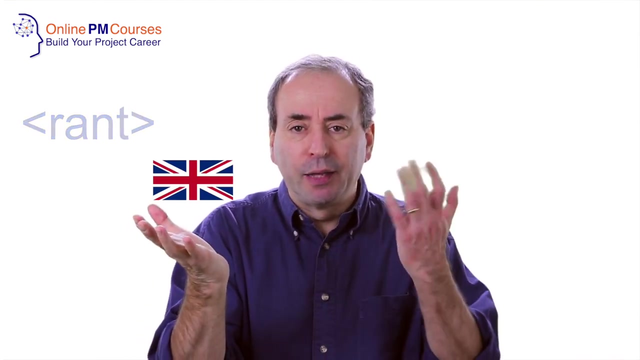 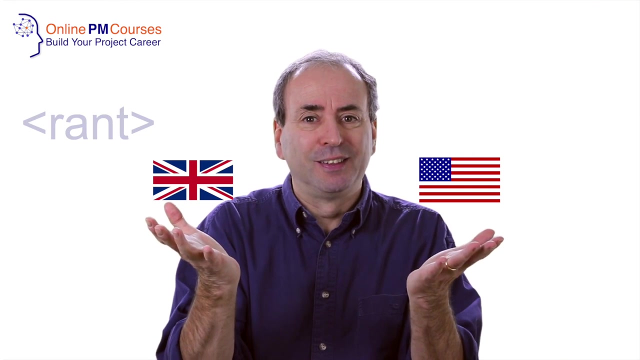 resources to carry them out properly. and i'm going to end with what is sometimes perceived as a bit of a rant. it's about the difference between the UK approach to work breakdown structures on the one hand, and the US approach on the other. neither is right, but here's the rant bit. 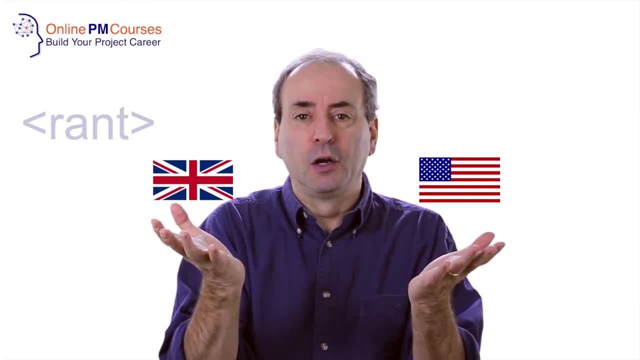 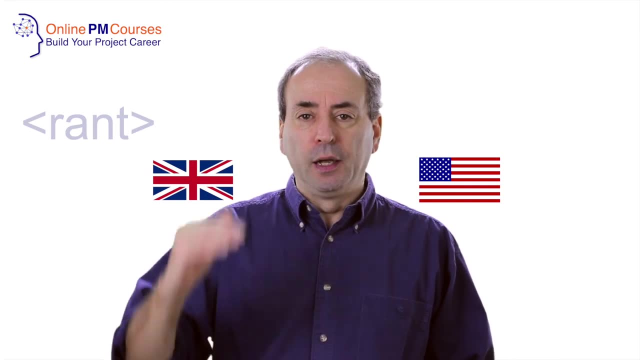 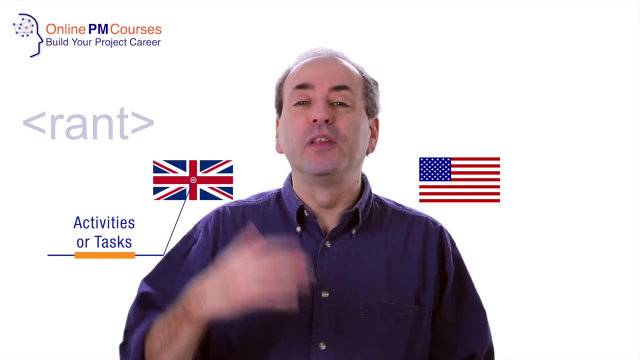 one of them is a little bit more right than the other. no clues. so in the UK our work breakdown structure is written as a set of activities or tasks. if you're a linguist, then you can think of them as written with verbs. the US approach is to break down the work. 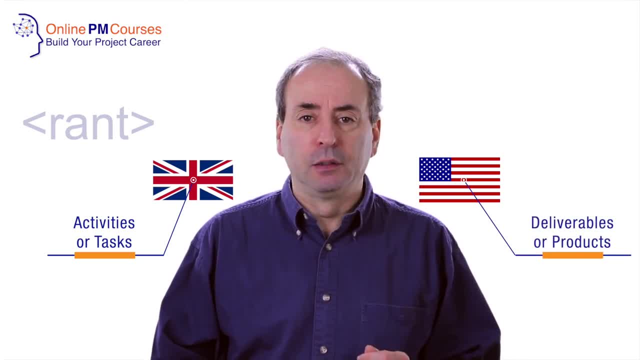 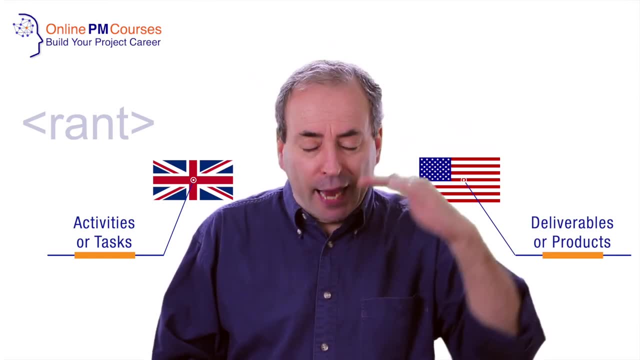 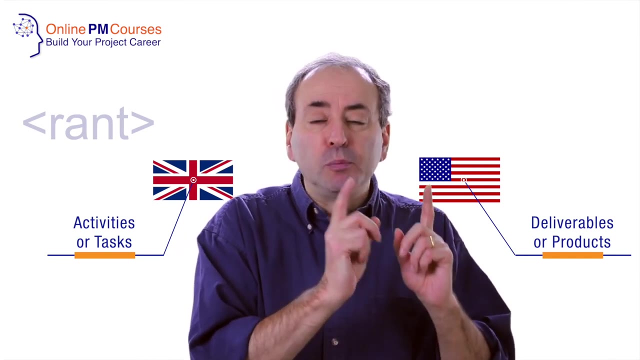 by breaking down the deliverables or the products for your project. so at the top level you have the completed project and at subsequent levels below you have more and more detailed descriptions and smaller components of the product set you need to create. in the UK we would call that a product. 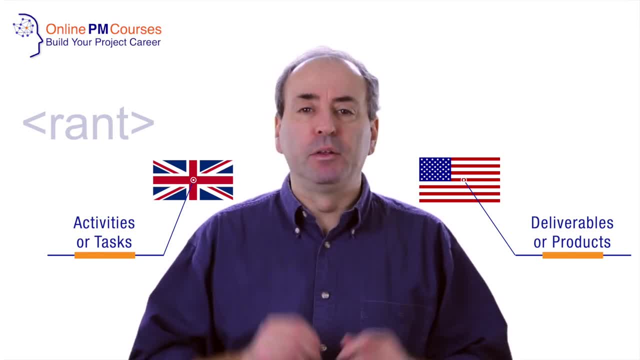 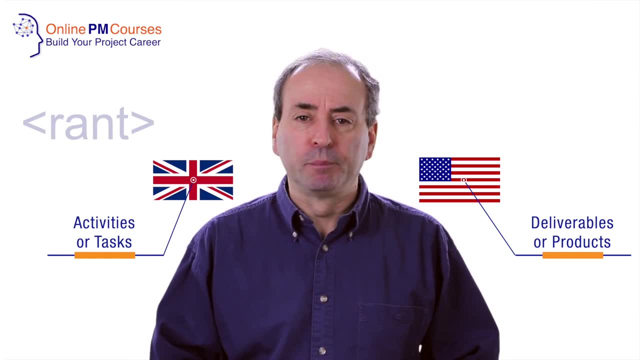 breakdown structure. both of them will give you the right results. so why do i prefer the UK approach? well, because it's a work breakdown structure that breaks down the work. if you want a product breakdown structure- and oftentimes you will, then you can create a product breakdown structure in parallel.